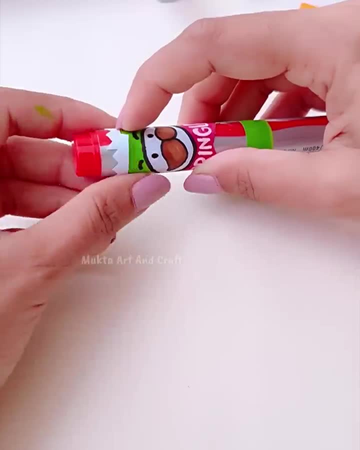 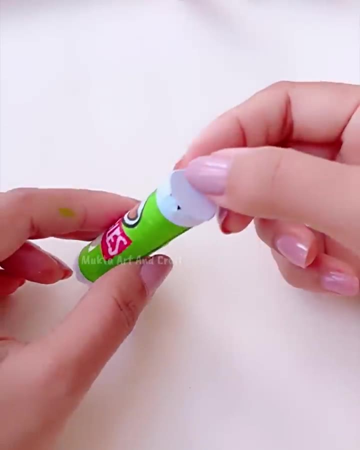 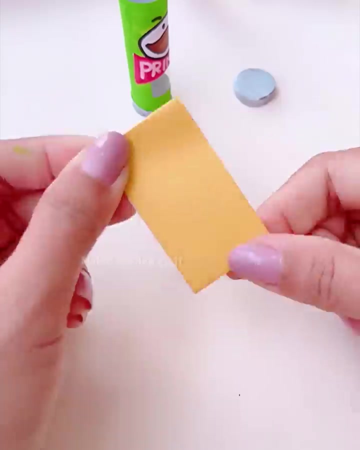 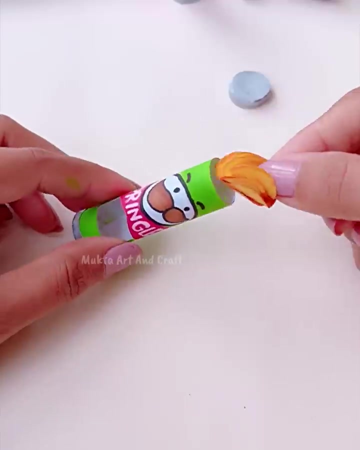 Baby boy, join me if you want to. We've got jumpsuits in glitter and red, Paper breakers and puppies in bed. We've got it all. tonight we pile up, We've got it all. yeah, If you ask, will I trust. I said maybe. 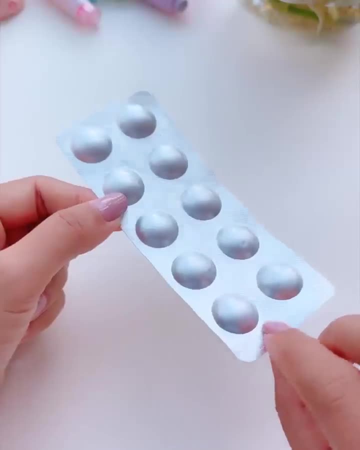 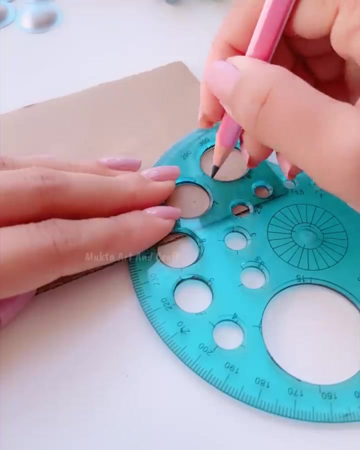 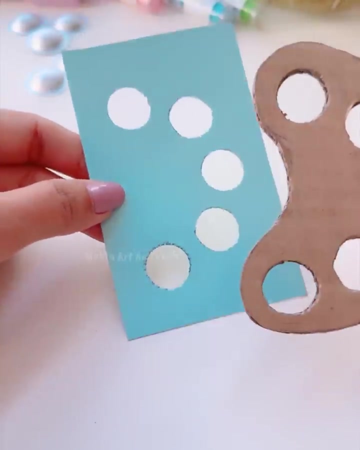 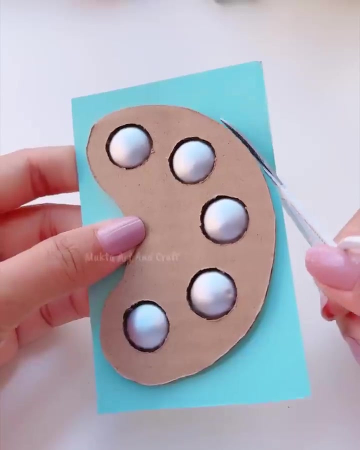 It's your call. Take a chance With this romance. I don't need lessons to see where credit catch. See my love's a vacation. I've been good and patient, But becoming real good, letting go. I can never fake this. I'm relentless in the metrics. Now it's time for you to show. 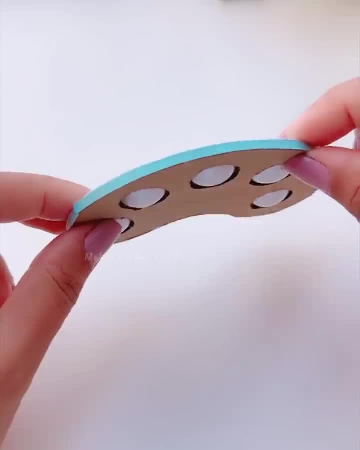 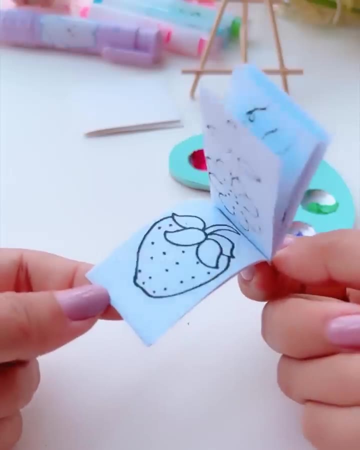 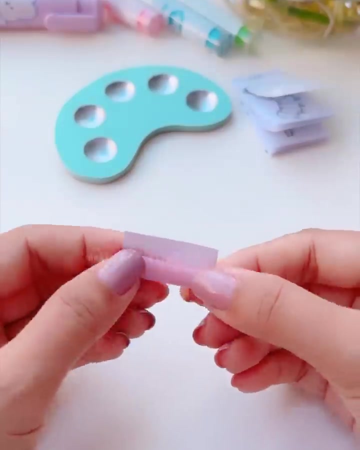 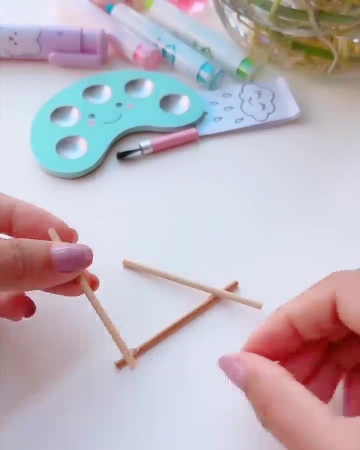 Living with passion. I love you. I live with stars. I keep my head steady, but feet are off the ground. I like it lush my lips so smooth. Baby boy, join me if you want to. We've got jumpsuits in glitter and red, Paper breakers and puppies in bed. 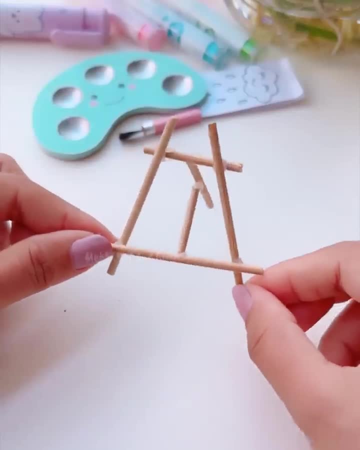 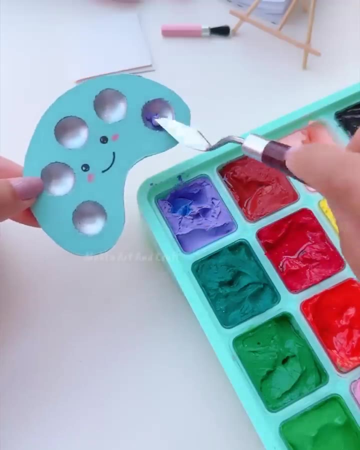 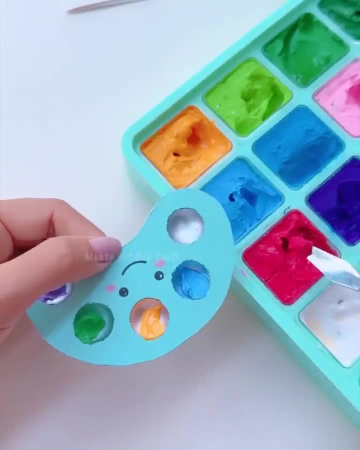 We've got it all. tonight we pile up, We've got it all. yeah, We've got it all. yeah, Baby boy, join me if you want to. Baby boy, join me if you want to. We've got this taste, We've got it all, baby. 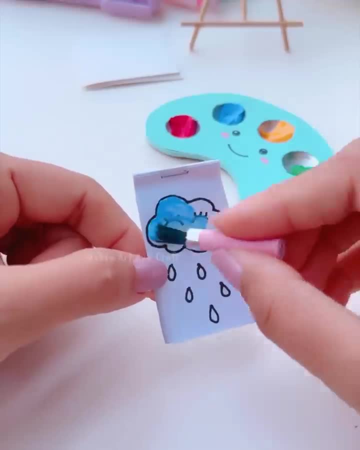 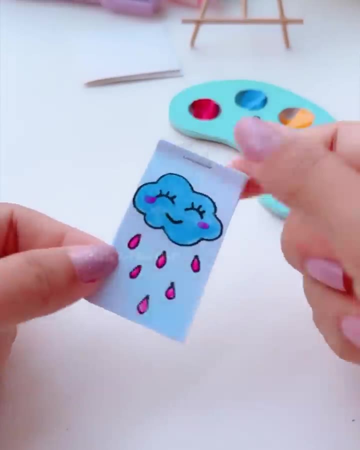 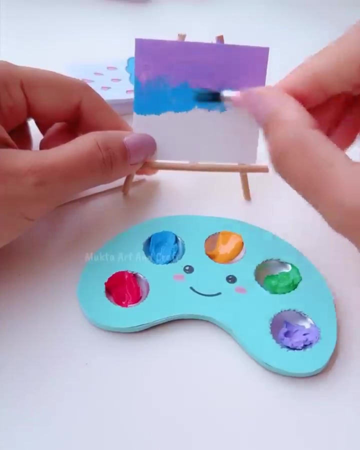 Take a chance. We've got it all, so why not Take a chance? We're on the go, We're on the run. Take a chance, We're on the roll. No more waiting, We're on the run, We're on the run. Be my Johnny if you want to. 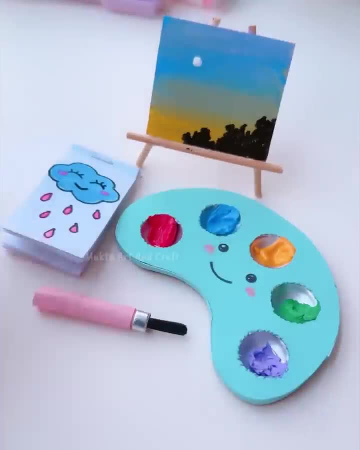 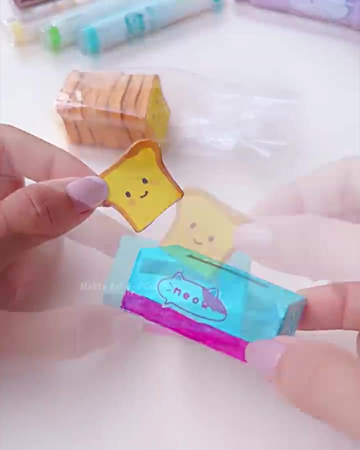 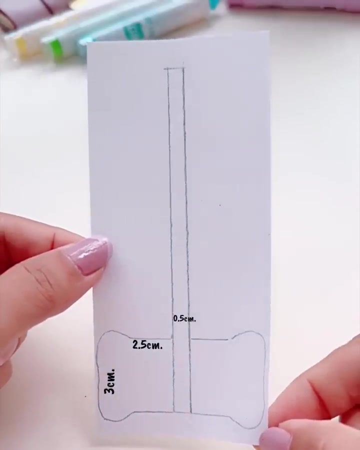 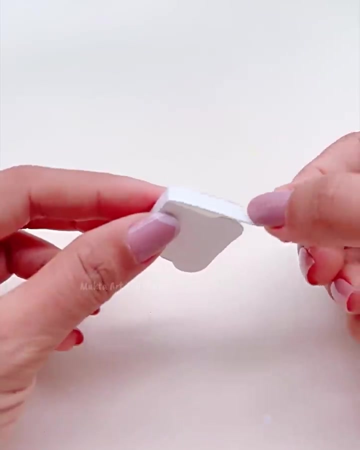 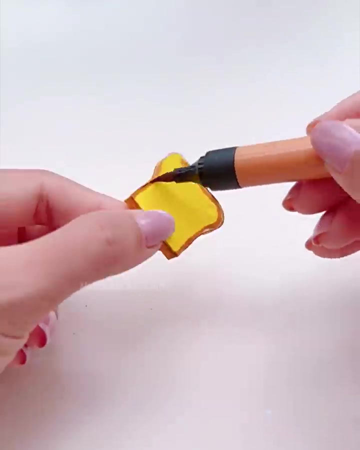 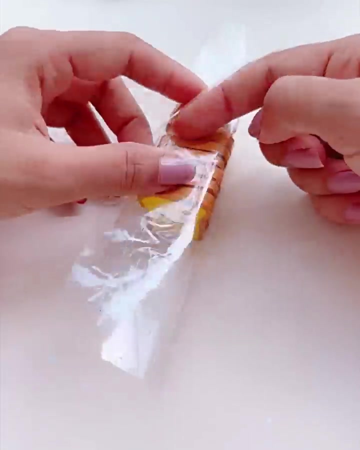 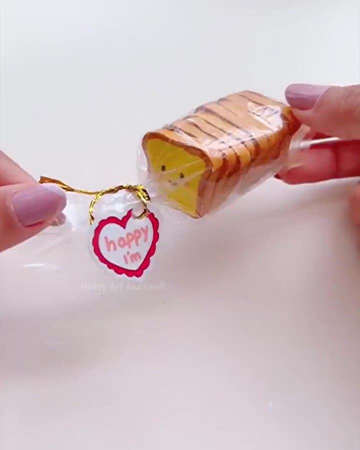 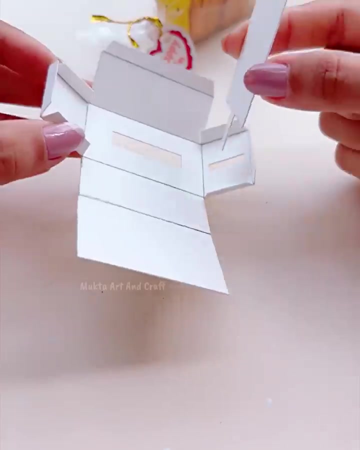 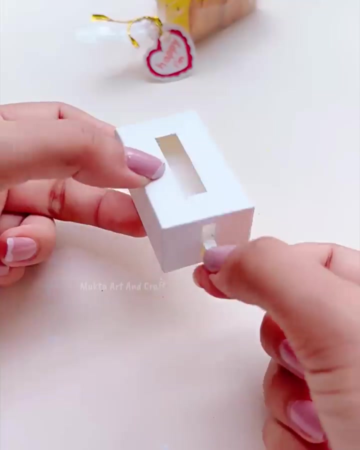 We've got it all. We've got jumpsuits in redder and redder. Take a breakfast and pop these in bed. We've got it all. Tonight, we party up. We've got it all. We've got it all. We've got nothing to say. You hold your head high. 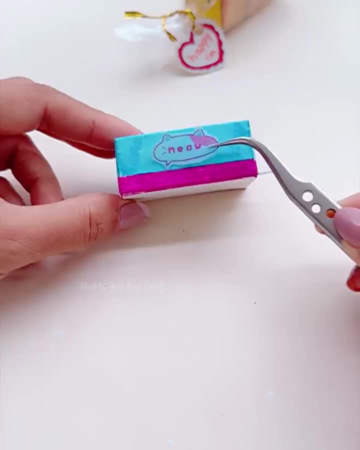 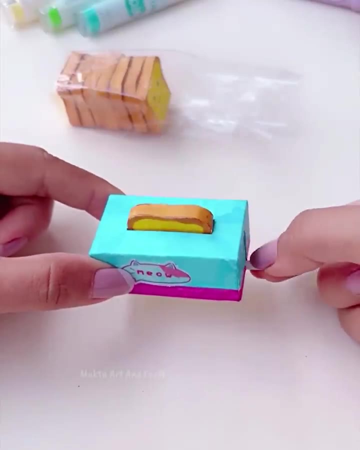 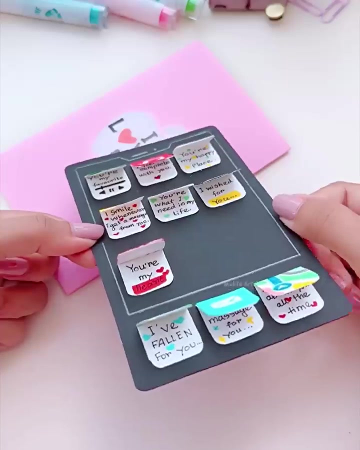 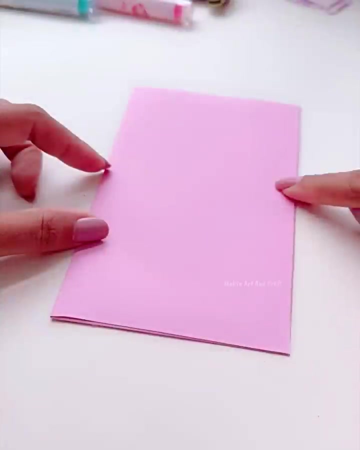 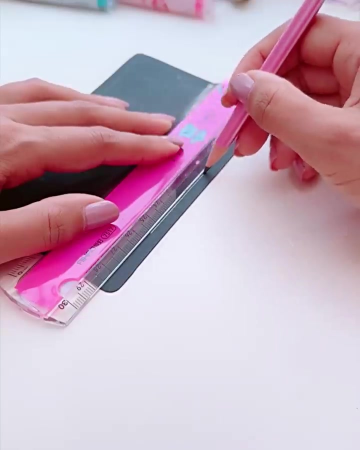 But your morals they fade. I know you feel cool, But your bubble will break, Oh well. oh well You can walk into a room And every fool Will try to be like you. But I'm not gonna sell my soul Just to be someone. you wanna know. Who you like is out of my control. 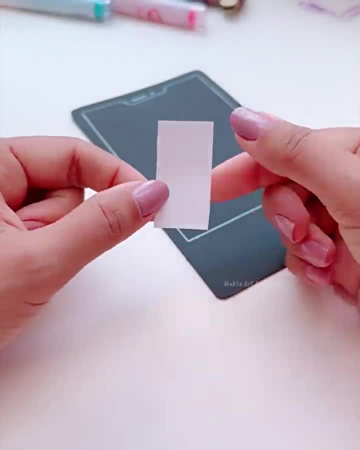 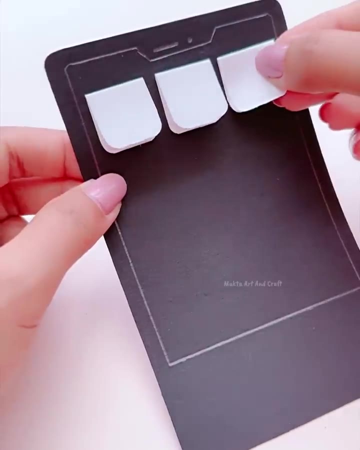 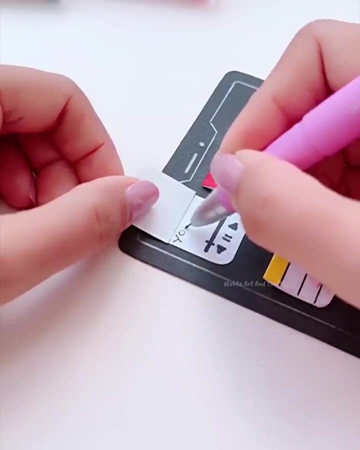 I'm okay being me. I'm not gonna change myself Just to make you fall under some spell. Rather be alone than be a shell. I'm okay being me. You say: you don't judge And you don't judge, And you don't judge. My friends all look great. 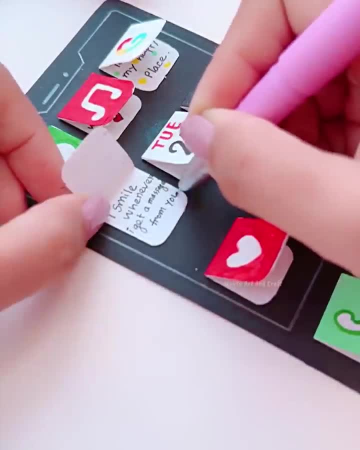 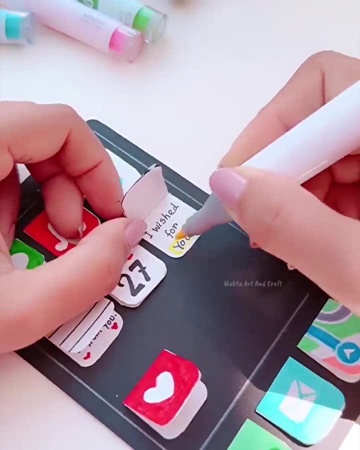 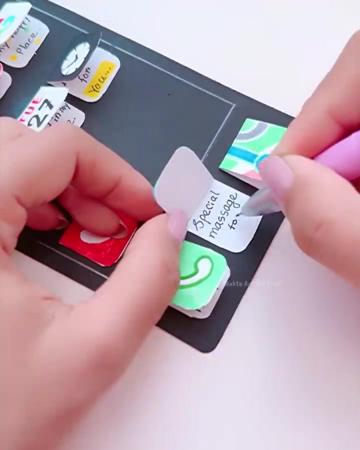 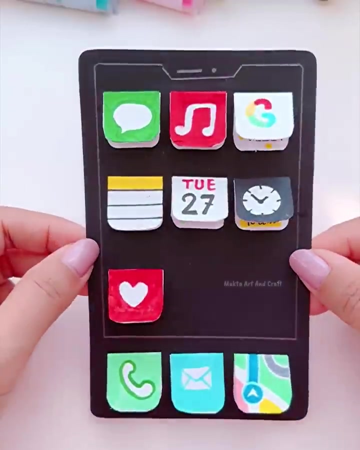 They see you fool you, But they don't see what I see: I'm a narcissistic personality. Oh well, You think the world is yours. You think it spins for you. You think you did some more Than every other fool. You can walk. You can walk into a room. 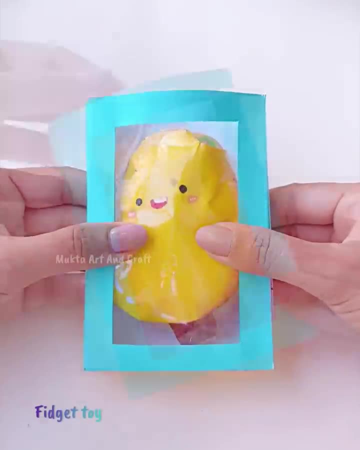 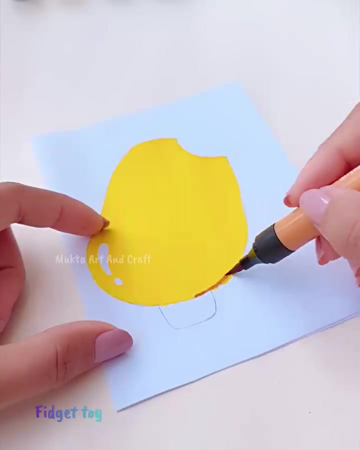 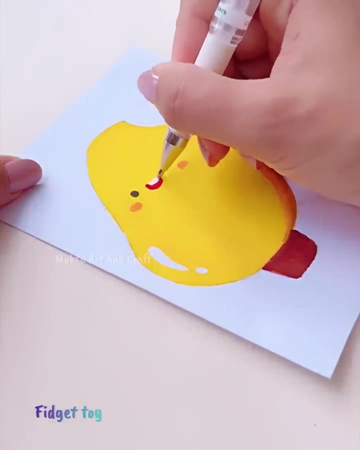 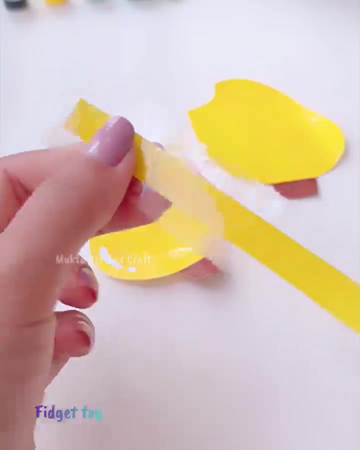 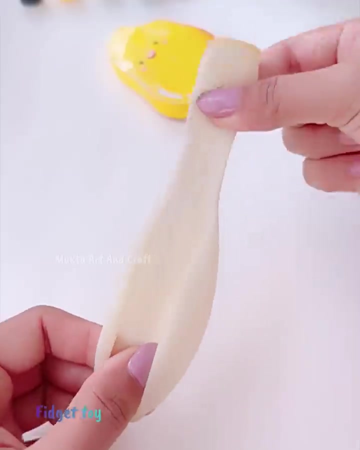 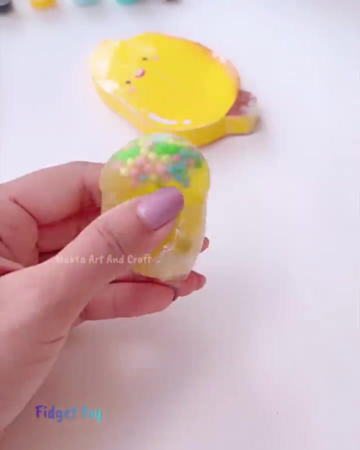 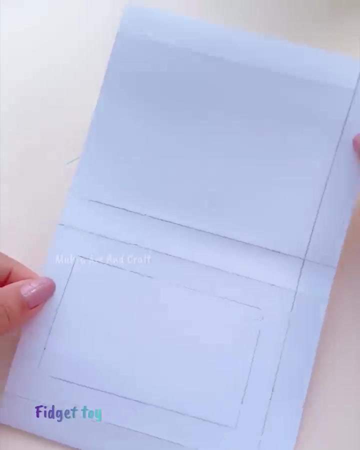 You can walk into a room And every fool Will try to be like you. You can walk into a room. I'm not gonna sell my soul Just to be someone you wanna know. Who you like is out of my control. I'm okay being me. I'm not gonna change myself. 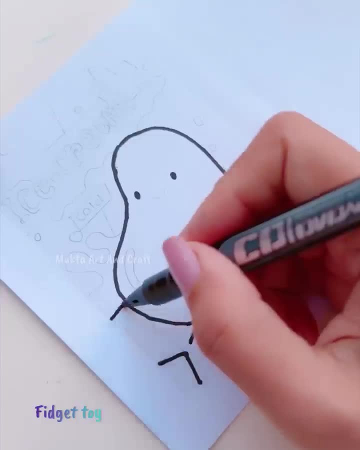 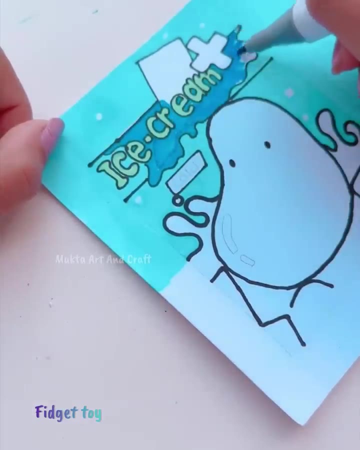 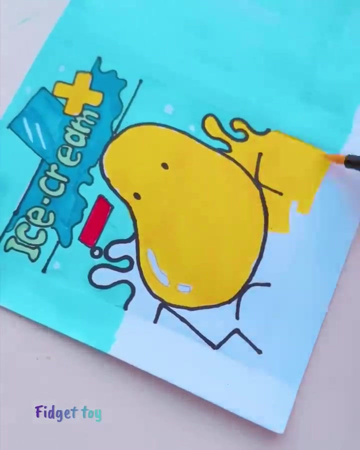 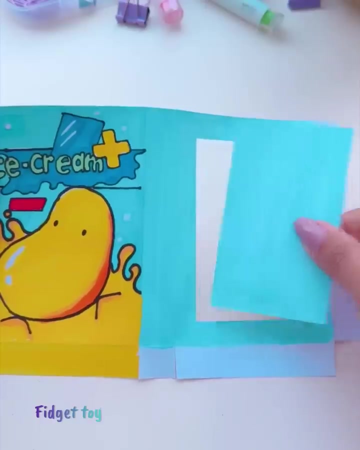 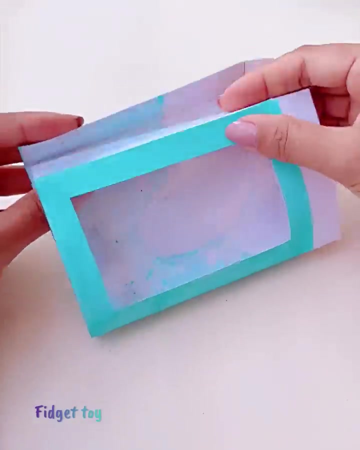 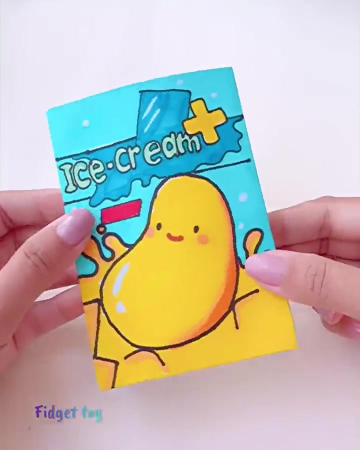 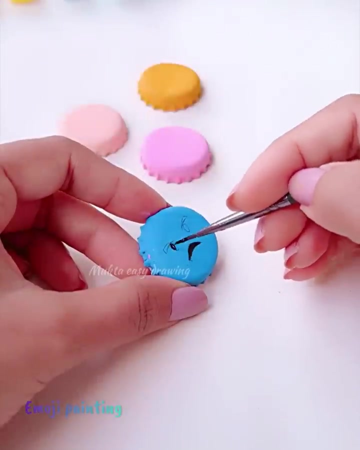 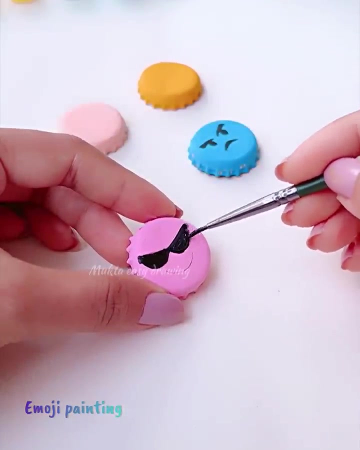 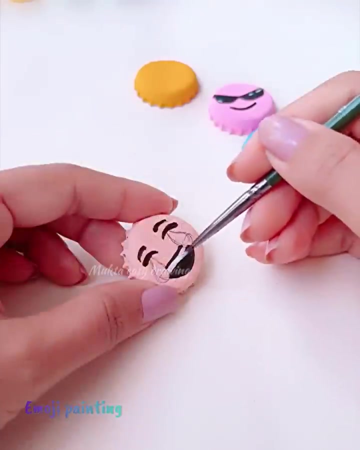 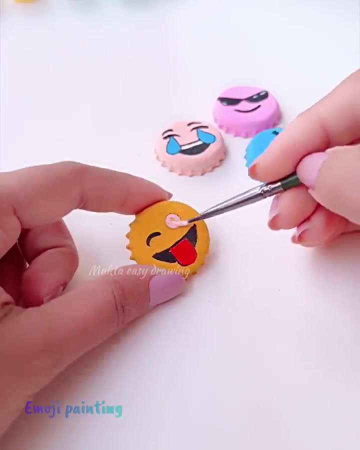 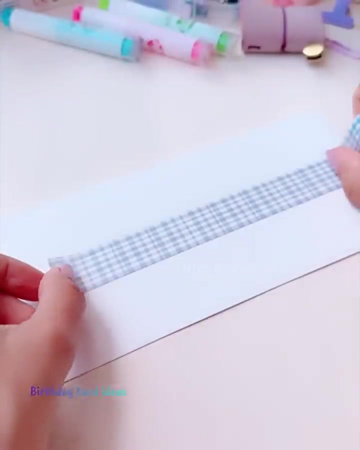 Just to make you fall under some spell. Rather be alone than be a shell. I'm okay being me. I'm okay being me. I'm okay being me. Posting every day, Making sure she's in every frame Who you're trying to impress, Telling everyone, including my friends. 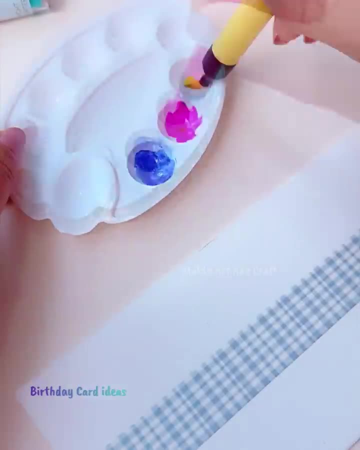 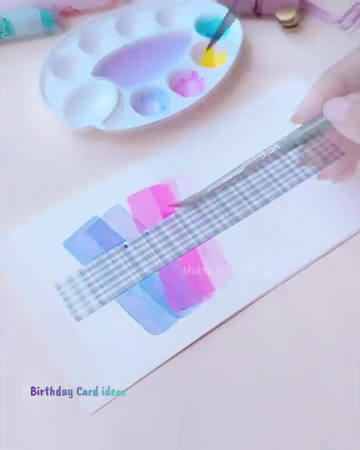 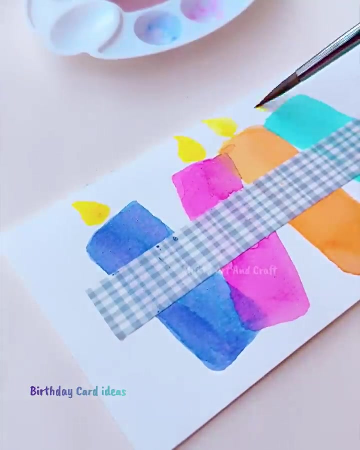 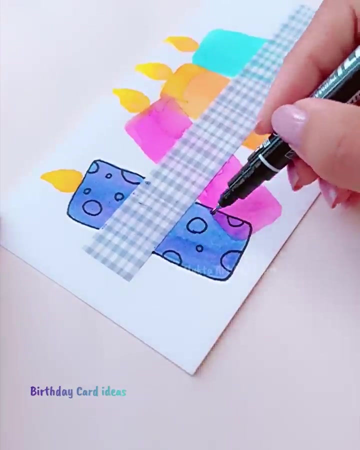 That she's the one Making sure I get the message. You always find a good excuse To show her off, But I've never been more over you, So you can't stop. Honestly, I don't care, I don't care, I don't care, care, care. 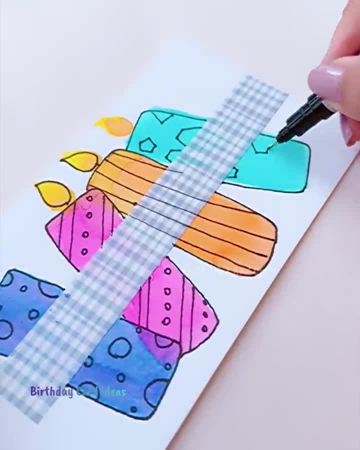 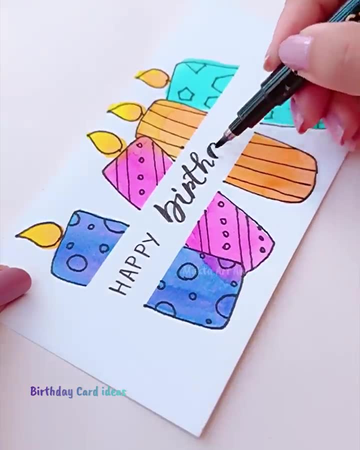 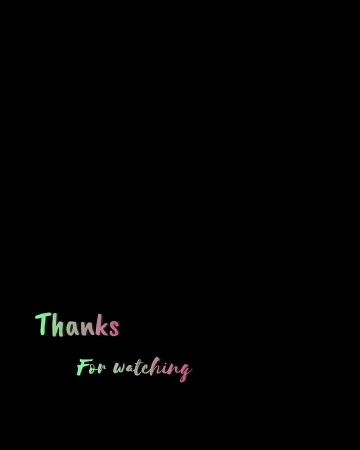 That she's cool, funny, too pretty. It almost seems to me You want jealousy, But please, there's no need. I don't care, Couldn't care less. I swear I'm in paradise, Do my thing, not thinking twice. Guess it hurts for you to see that.